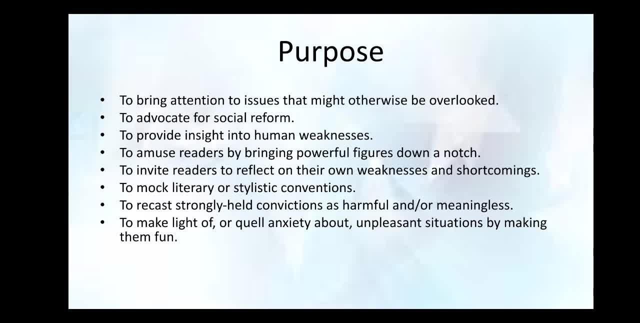 stupidity, some agency's stupidity or some weakness. we actually advocate that particular problem of society in front of the readers. to provide insight into human weaknesses, to amuse readers by bringing powerful figures down a notch, to invite readers to reflect on their own weaknesses and shortcomings. so we see satires not only reflect on the weaknesses and flaws of others, but also on one's. 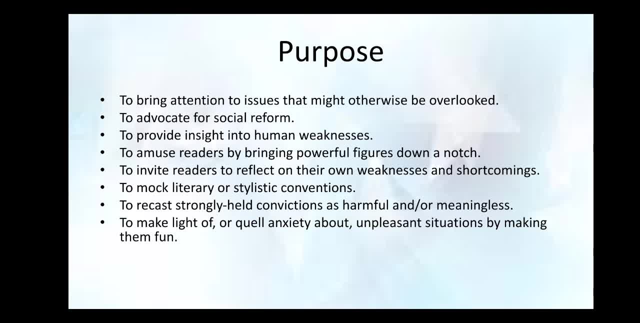 own universal or human weakness or shortcoming that we may not actually look into without reading these words. then, to mock literary or stylistic conventions, the old traditional setups that have already carried on for the past few centuries or decades we generally tend to overlook. but through a satire, 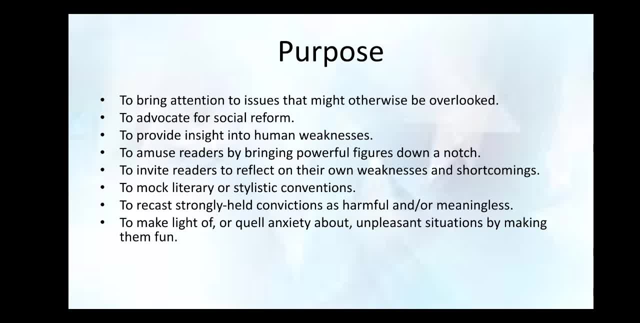 it is to mock those stylistic conventions that have been set up and that now need to be broken or changed. then to recast strongly hand convictions as harmful and meaningless, to make light of or quell anxiety about unpleasant situations by making them fun. so basically, satire, we see, is a. 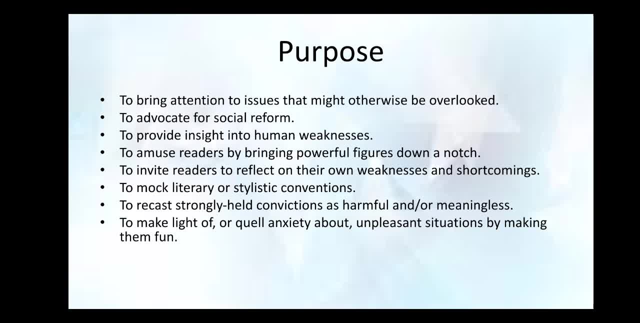 form of writing that uses the tools of humour, irony, exaggeration or ridiculing to get into light or to uh quell or satisfy the anxieties about certain situations which are unpleasant or which evoke curiosity, or they are enigmatic. vis γκννangle Influenced Orų Carroll Either One or other Aspect nesse. 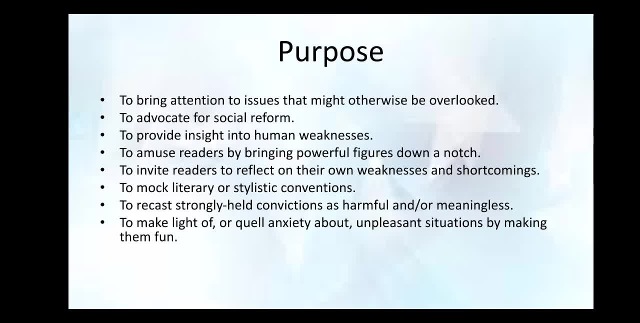 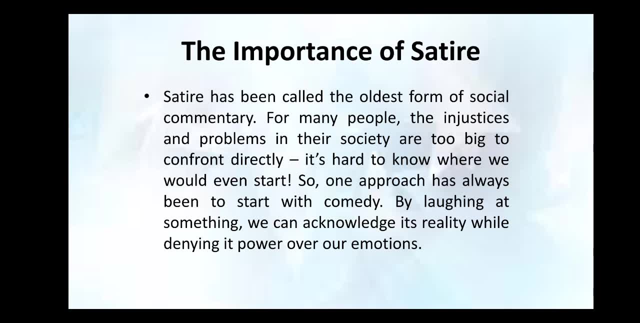 directly address those situations, but through satire we are able to look at those situations in a different light. Now, it has played an important role throughout the history of English literature, and satire has been called the oldest form of social commentary. For many people, the injustices and problems 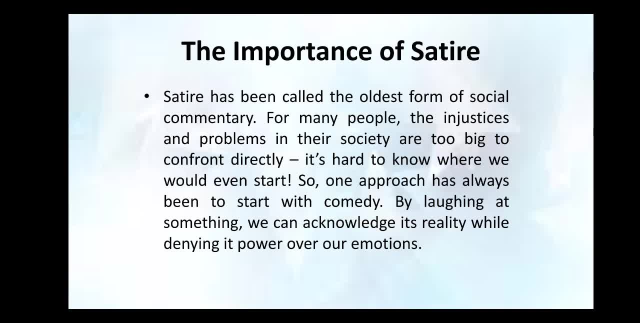 in the society are too big to confront directly and it is hard to know where would we would even start. So one approach of handling and confronting these problems of society has been to start with the comedy. By laughing at something, we can acknowledge its reality while denying its power over our 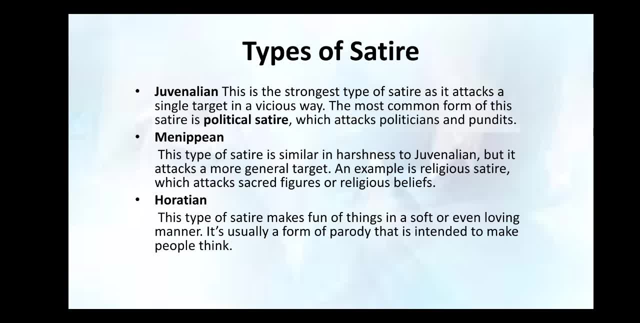 emotions. Now we have different types of satire. satire is not just a one-kind. we have the juvenal satire, which is the strongest and you can say the bitter beyond words. To relax and take on mental well-being is very important. most type of satire because it attacks a single target in a vicious way. you know. 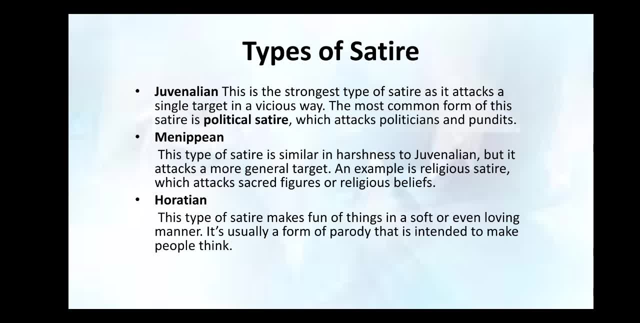 in a kind of a negative light. and the most common form of the satire is political satire, which actually attacks politicians and pundits and the great diplomats of a nation, of or of a place. then we have the Minipian. now this satire is somewhat similar in harshness to jubilant, but it attacks a more general 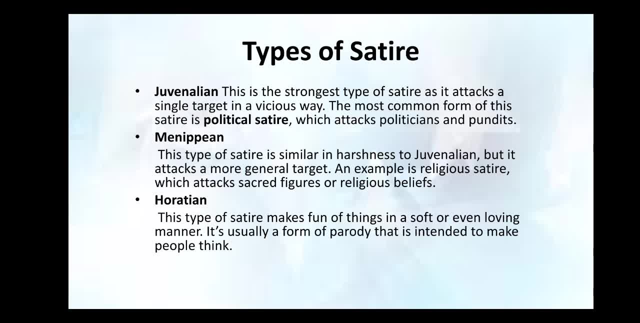 target. so general means it can be an institution, it can be a set up, it can be a community. for example, we have the religious satire. so this one religion could be a target, one church could be a target, one community could be a target which attacks sacred figures or religious beliefs. so it is more. 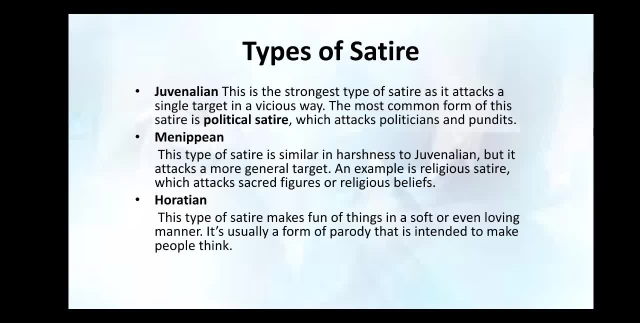 generalized, a group community kind of the satire community kind of a thing being targeted. then we have Horatian. this time it's a satire which is a group satire. it's a satire which is a group satire of satire. makes fun of things in a more soft or even loving manner. it's cool. so it's usually a 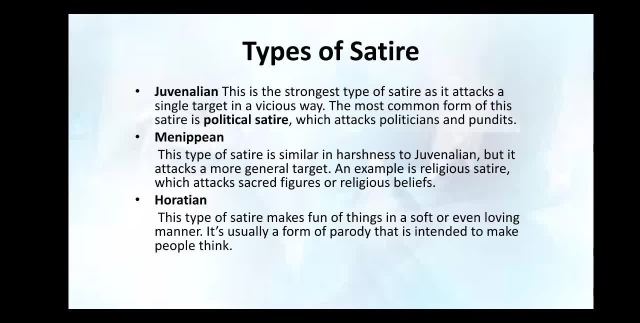 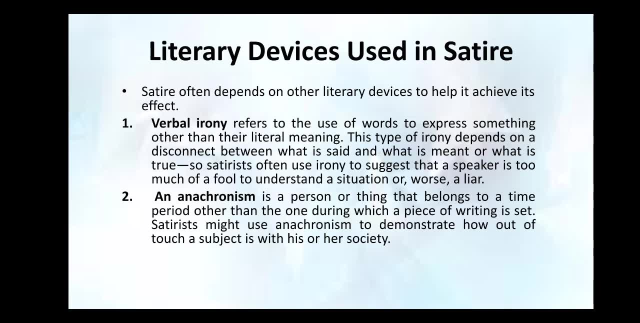 form of parody which is intended to provoke the thoughts of people. it is. it intends to make people think about something particular which is not suitable or unpleasant in society. now, how does satire build itself up? where does satire stand? does it stand on its own? no, it does. it does need. 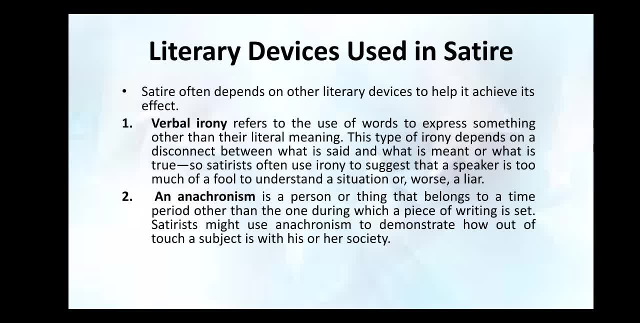 the help of literary devices to achieve the effect that it wants to. maybe it is humor, maybe it is sarcasm, maybe it is understatement. overseeing something exaggerates exaggerating something. so we briefly talk about the devices that it takes the help of while building up. so 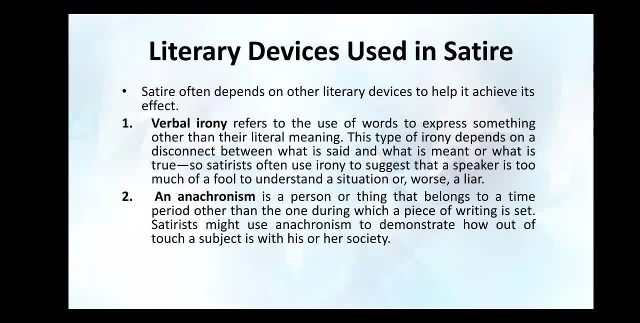 satire often depends on other literary devices to help achieve its effect. so the first is and foremost device, which is mostly and generally used in all kinds of satires, is verbal irony, and irony refers to the use of words to express something other than their literal meaning. the word that we are using may not literally mean the same, but would in fact imply something. 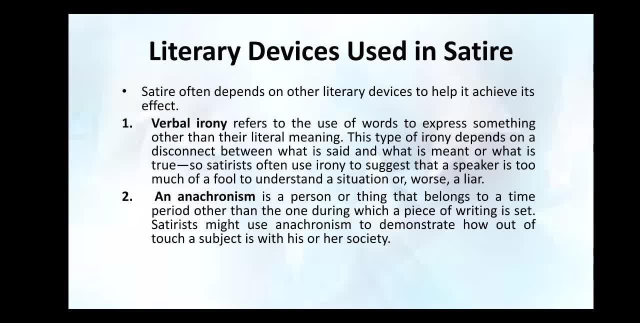 else would target at something else or hint at something else that we want to say now. this type of irony depends on a disconnect between what is said and what is meant, or what is meant and what is meant what is true. so satirists often use irony to suggest that a speaker is too much of a fool to 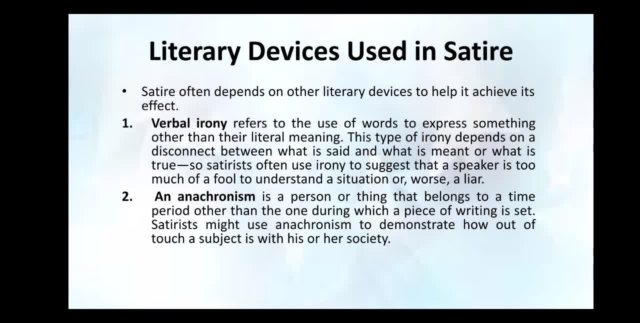 understand a situation or, worse, a liar. so this is something that we use to imply something else that we want to say, but in a soft tone, using a very soft literal word, which may imply something harsh or unpleasant, or unwanted, or exactly the opposite. then we have the tune of anachronism. 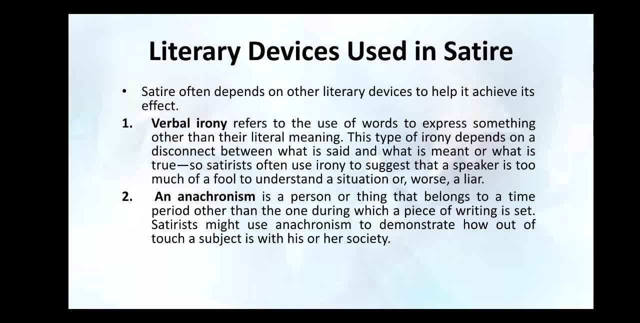 now, anachronism is a person or a thing which belongs to a time period other than when we are writing. when the piece is being written, satire is being written, so something related to another period, another age, another time. satirists might use anachronism to demonstrate. 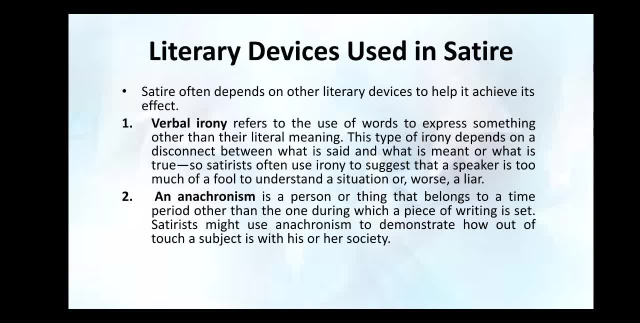 how out of touch a subject is with his or her society. for example, in this age of science and technology, we we just talk about lighting a fire, or we talk about moving out, or carts, bullock carts and all that, and we think of a civilization without roads. so it goes out to a 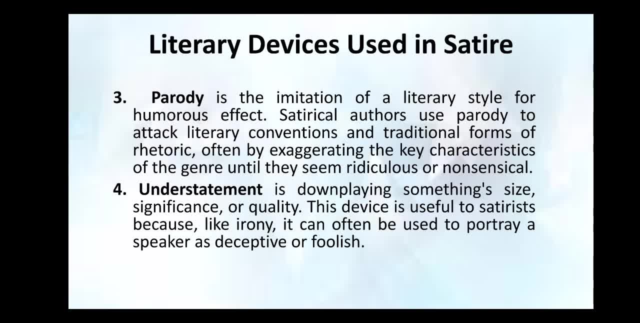 time which does not match with our own time. then we have a device called parody, and parody is the imitation of a literary style for humorous effects. so normally when the authors write satires they use parody to attack the literary conventions and the traditional forms of the rhetoric, often by the 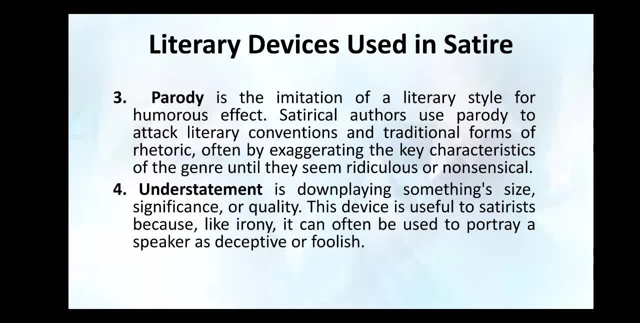 use of exaggeration, exaggerating the key elements, key characteristics of this genre until they seem ridiculous or absolutely nonsensical. then we have the understatement. understatement is like when you say something lesser than what you want to convey. it is downplaying something's size, significance or quality. now this actually device like irony can be used to portray a. 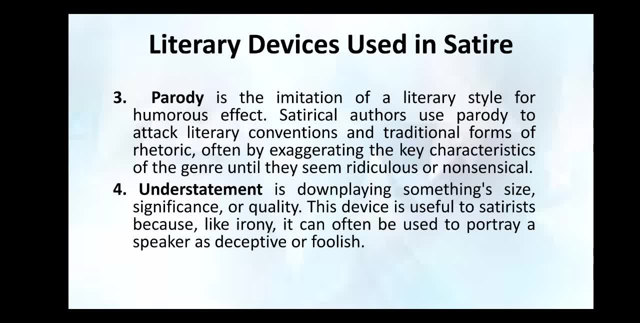 speaker as foolish. for example, a speaker is saying something which actually should have a lofty or a big meaning or a big use of language, but he is using very simple or lesser words to just give the impression that he is foolish or he doesn't know the thing or he is being deceptive. so this is 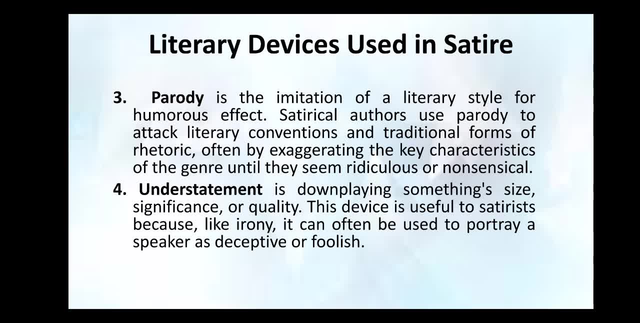 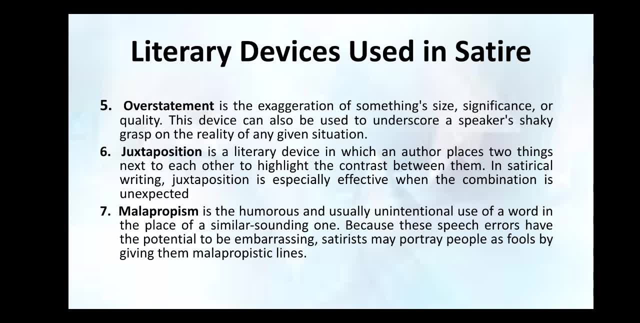 understatement, saying lesser than what is required. then we have the overstatement. overstatement is the exaggeration of the word understatement. understatement is the exaggeration of the word understatement of something which is actually looking like, something which is actually seeming something size, significance or quality. now this device can also be used to underscore a person's shaky grasp. 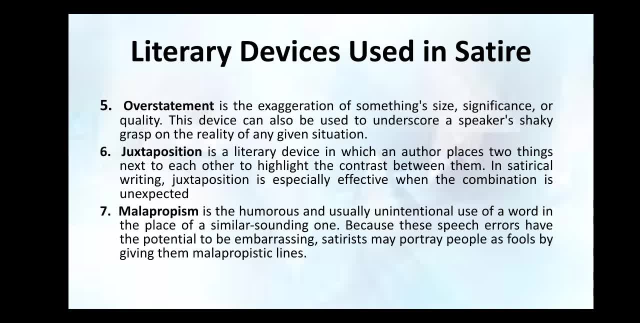 on the reality of a given situation. for example, if the writer wants to say something and he is over exaggerating his idea or his point, or something is being over exaggerated which gives the impression that he is shaky, he does not have a grasp on his topic or his point, then we have the juxtaposition. 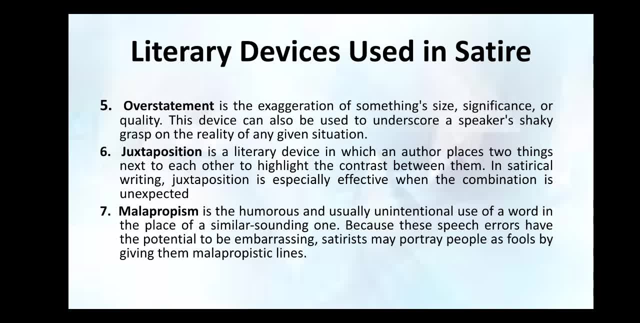 where we have comparison of two things, in which the author places two things next to each other to highlight the contrast between them. so basically, it is a parallel, it is a comparison, and in satirical writing, juxtaposition is especially effective when the combination is far-fetched. it is not expected. 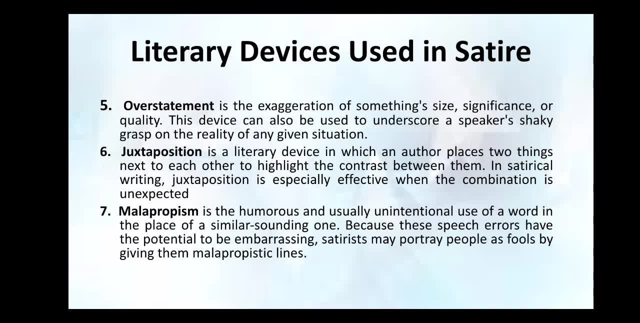 by a common reader and it is unexpected, then. malapropism is the humorous and usually unintentional use of a word in the place of a similar sounding one. now, because these speech errors have the potential to be embarrassing now when you use the word actually, you wanted to. 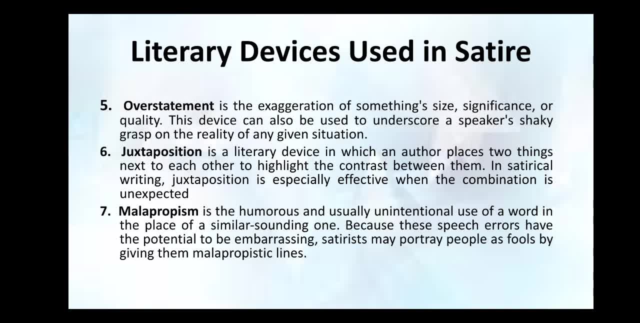 use some other work, but because of slip of tongue or an unintentional mistake, you use another word. so, for example, it is ruler and you say rule, or it is rule, you say ruler. so kind of confusing that what you want to say could not be conveyed properly. and these are speech errors which 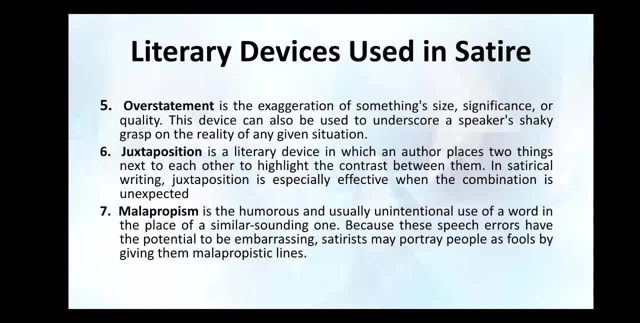 make you embarrassed as writers, as speakers. so satirists may portray people as fools by giving them malapropastic lines. so when you miss, misspell, mispronounce or you give an error in your speech to the audience, you sound foolish. so what satirical writers used to do? 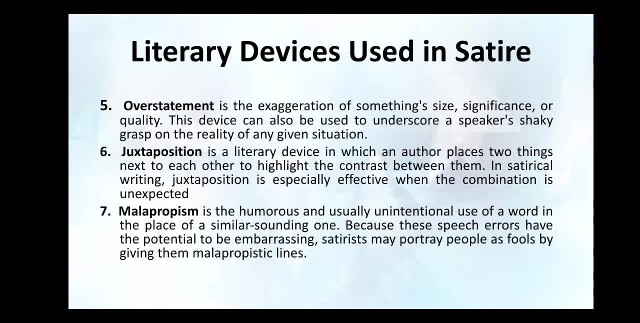 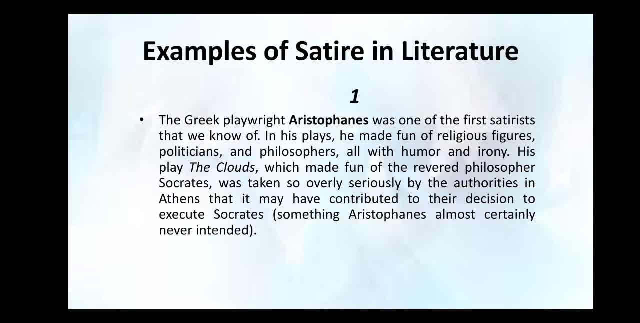 was. they used to give these malaprophastic lines to speakers or characters whom they wanted to look foolish. now I'm an important part to understand this concept of satire, in which we see that the whole work is a satire. we should study the examples of satire now. the first satire: 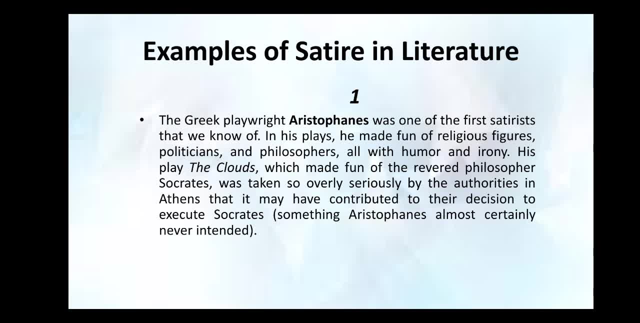 is that of, was the Greek playwright Aristophanes. In his plays he made fun of religious figures, politicians and philosophers, all with humour and irony. His play, The Clouds, which made fun of the revered philosopher Socrates, was taken so overly serious by the authorities and atheists. 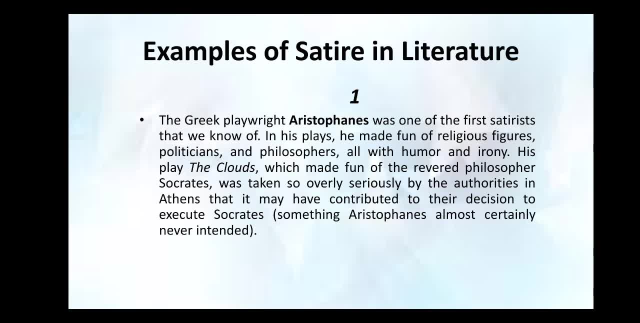 that it may have contributed to their decision to execute Socrates, Although we came to know that Aristophanes never intended that his writing on Socrates would lead to such drastic or negative results. So we see Aristophanes writing. the play actually showed Socrates in a. 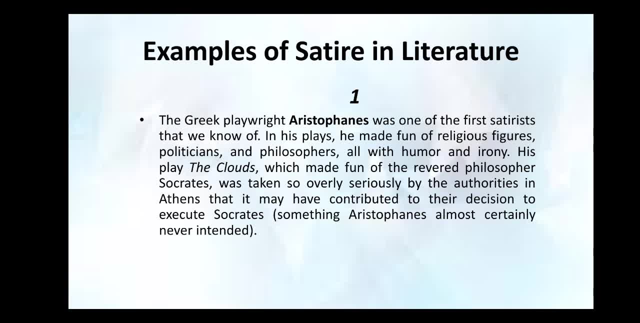 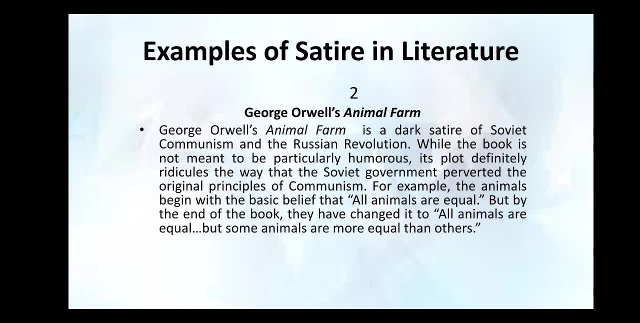 satirical light, so much so that the impression of the society about Socrates changed. Then we have a very popular example of satire- The whole work is satirical- and that is George Orwell's novella Animal Farm. Animal Farm is a dark satire of Soviet communism and Russian revolution. 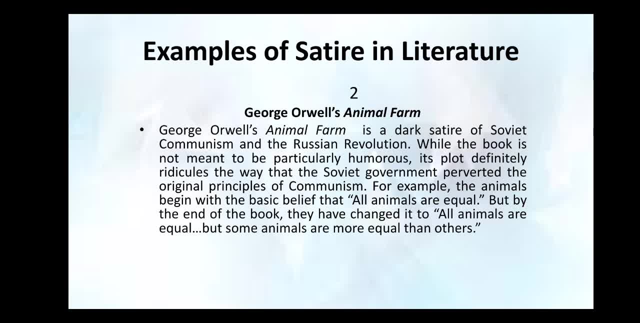 While the book is not meant to be particularly humorous, its plot definitely ridicules the way in which the Soviet government perverted the original principles of communism. For example, all the characters in this novella are animals, And these animals begin with a basic belief: that all 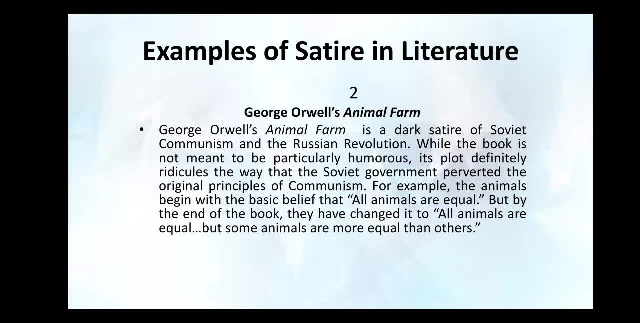 animals are equal, But we see as we move in the novel, by the end of the book they have changed it too. All animals are equal, but some animals are more equal than others. Now, this is highly, highly humorous, ironical and satirical. 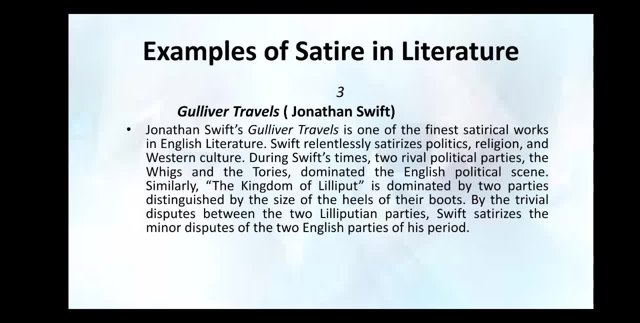 Then again we have another very popular, famous and very popular novel: The Clouds. The Clouds is a novel by George Orwell. The Clouds is a novel by George Orwell. The Clouds is a novel by George Orwell. Now, this is also one of the most ever-famous and well-known work by Jonathan Swift, which is the Gulliver's. 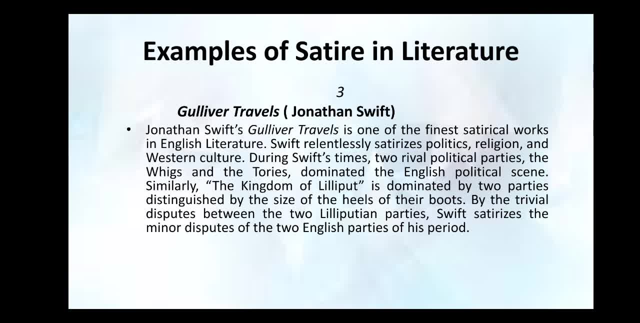 Travels. Now this is one of the finest satirical works, the most quoted in English literature, Because Swift relentlessly satirizes politics, religion and Western culture. Now, during his times, there were two rival political parties, the Whigs and the Tories, which dominated the 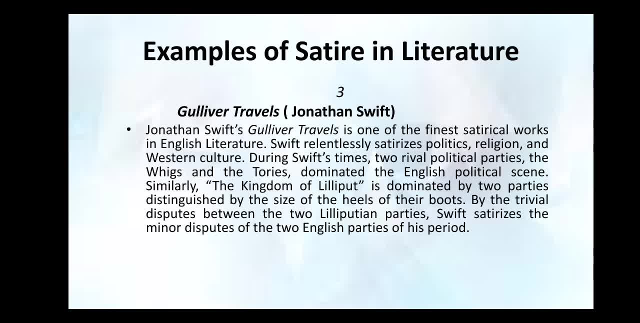 English politics. Similarly, in his we see the kingdom of Lilliput is dominated by two parties distinguished by the size of heels of their boots, So by these small, mundane, tricky and trivial disputes between the two Lilliputian parties. Jonathan Swift satirizes the minor disputes of the two English parties of the 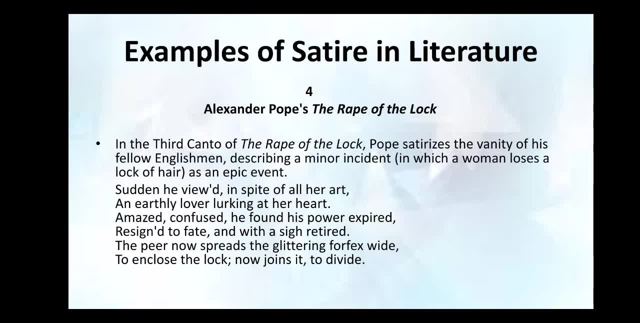 period, Then another fine example of satire that we usually study in our postgraduate classes also is Alexander Pope's The Rape of the Lock. Now, this play is a complete satire in more than one sense. For example, in the third canto of The Rape of the Lock, Pope satirizes the vanity of 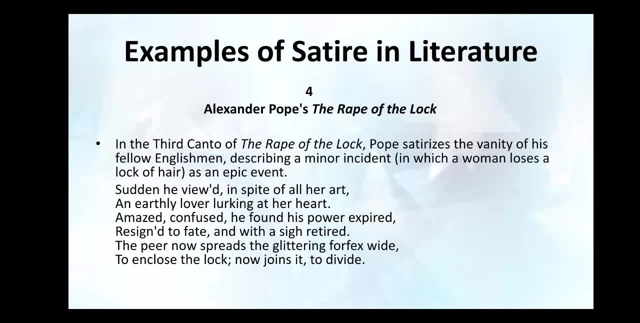 his fellow Englishmen describing a very minor incident. Now, this minor incident: if we have read The Rape of the Lock, we know that in this the woman loses a lock of hair, and which has been enacted as an epic incident. Suddenly he viewed, in spite of all her art, an earthly lover lurking at her heart, amazed, confused, and he found his power expired, Resigned to fate and, with a sigh, retired. the peer now spreads the glittering forefix, white to enclose the lock, now joins it to divide. 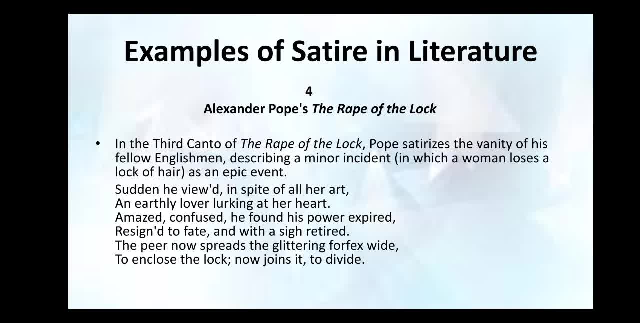 Now here what Pope is doing is. Pope is alluding to a real life episode In which Robert Petraeus stole a lock of hair from his love interest, Arabella, And Pope has successfully satirized the minor event by inflating its importance increasing. 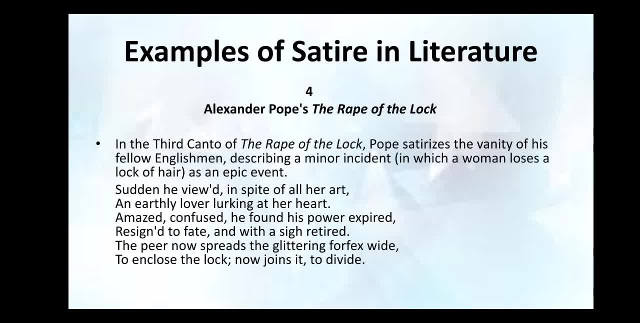 its importance to such an epic proportion. He makes reference to sylphs, which are mythological creatures which intervene in moments of crisis. He also overstates the male lover's frustration and also the extent to which fate played a role in the incident. The incident is the minor theft of a single curl, a lock of hair. 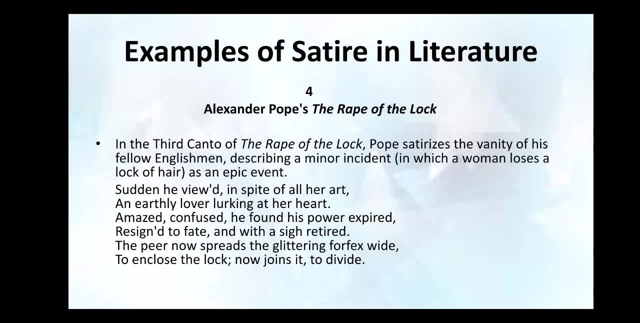 Then the repetition of like forever, forever in the final line also heightens the humor in the situation And obviously the hair will grow back in a short amount of time. But these lines are gentle jabs at his peer's fixation on appearances. So this becomes a very, very rich example of satire. 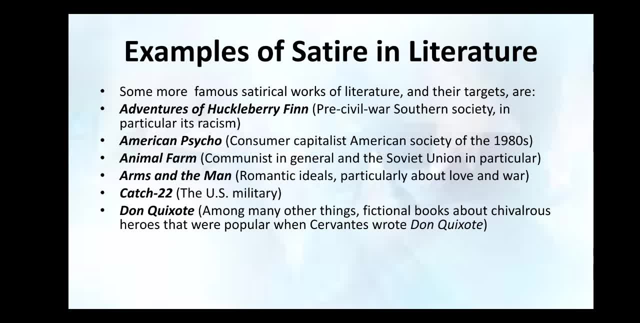 We may quote some more examples of satire in English literature. Some of these important examples are ''Adventures of Huckleberry Finn'', which targeted the pre-Civil War, Ukrainian anymorecancer, racism andLY. Then we have the American Psycho, which was targeting on Consumer Capitalist American society of bueno, why not? atBaba je be a代 nice digge d flips on me. 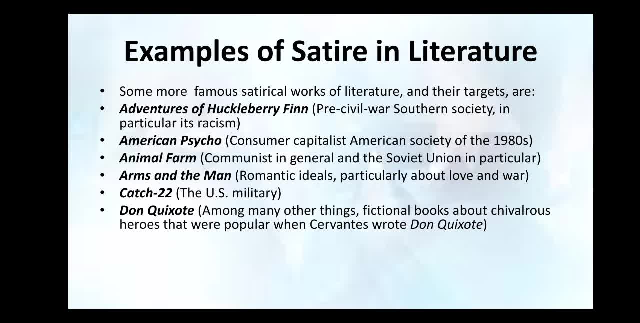 We have the American Psycho, which was targeting on Consumer Capitalist American society of bueno, where actually in actions berai tine us 그런데PAj walking behind a to Jay make other Speed to trespass 자 1980s. Then we've already talked about Orwell's Animal Farm. Then we have The Arms and the Man.